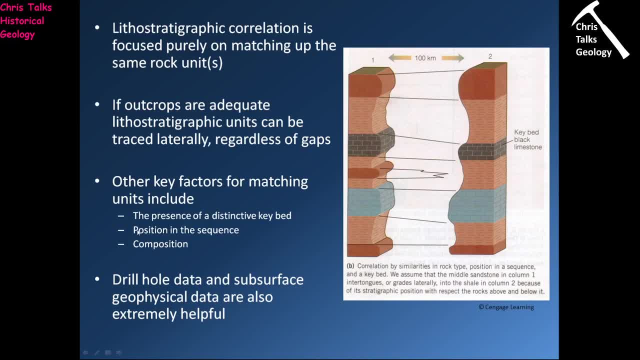 So the factors that, So the kind of things that we're looking for to begin with, is: are there any layers of rock which are distinctive? OK, so in a perfect world, what we want is some layer of rock that has something very, very interesting about it, something that stands out compared to the rest of the sequence. 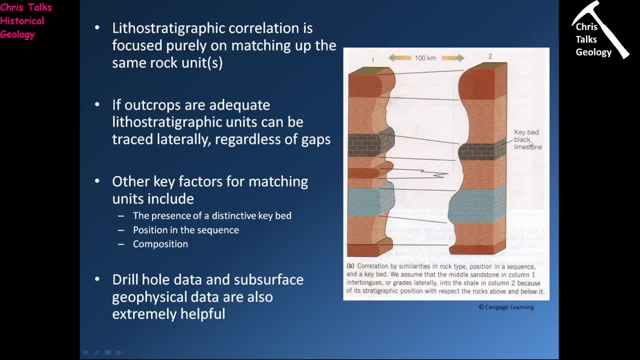 So we can see at these two locations, we have this layer here which is a black limestone. It's a very organic, rich limestone, And black limestones aren't hugely common, So when you see one in your sequence of rocks, it really catches your attention. 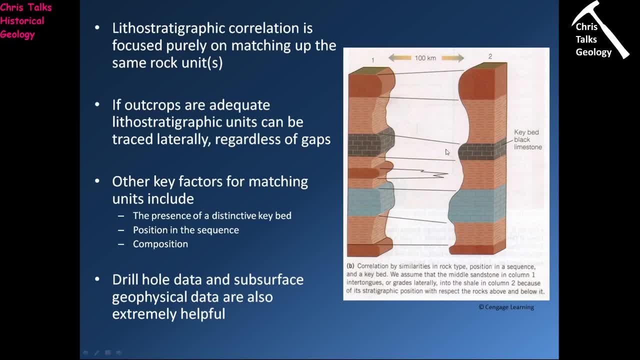 And so, because black limestones aren't, you know, hugely common rocks, you can use it to link up the two locations, because chances are, the black limestone you see at location two is the same black limestone you saw at location one. The other thing we can do is we can also use position in a sequence. 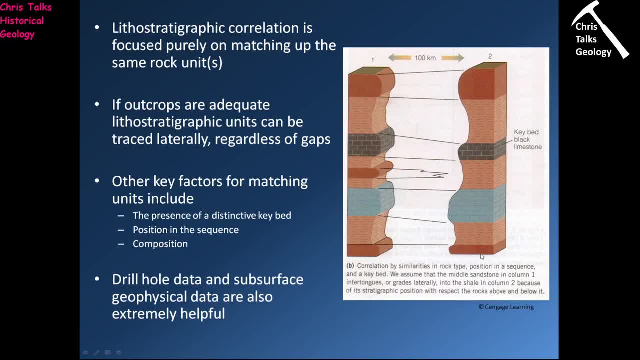 So we can see that at location one we have a sandstone, we have a mudstone, we have a limestone, we have another mudstone. Now this sandstone layer clearly pinches out somewhere. So between the two we have the black limestone we were just talking about, we have a mudstone, and then we have another sandstone. 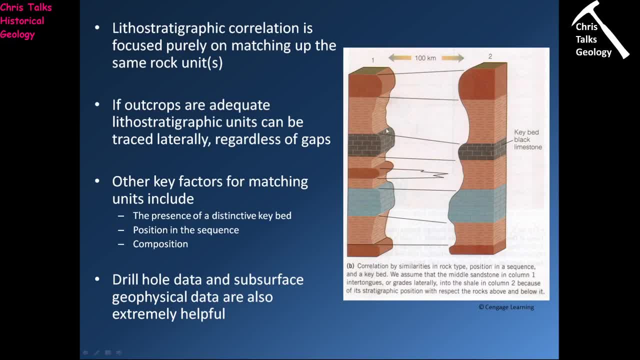 So, providing we know the sequence at one location, we can then look for the same sequence at the other location. And so, even if we didn't have the black limestone here, we would know it would go: sandstone, sandstone, mudstone, limestone, mudstone. 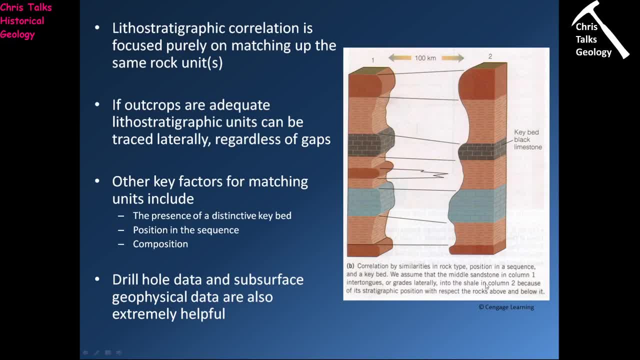 We're just going to say there's a normal limestone here, mudstone, sandstone. And if we saw the same sequence at location two, which we do- sandstone, mudstone, limestone, Mudstone, sandstone. sorry, getting a bit confused there- we can say, right, well, the position in the sequence is the same. 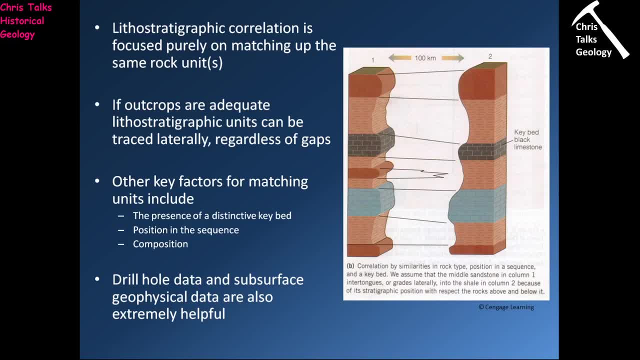 They match up. We can see the same layers of rock occurring in the same order, So we can once again correlate between these sequences of rocks. The final thing we can do- and this one is the most risky- is we can use the composition of the rocks. 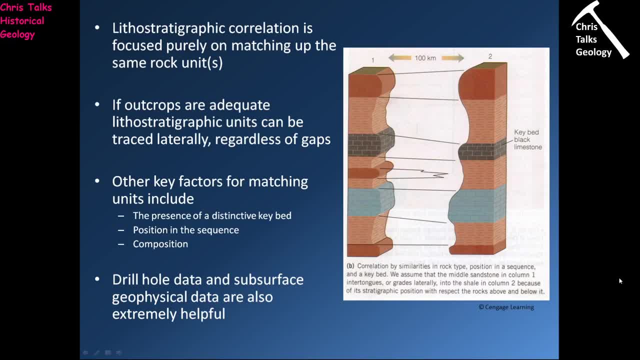 What are the rocks made from? Now, this one is dangerous. The reason is is that rocks will change in color, They will change in composition over, you know, laterally. So you know, this sandstone here may be 50% quartz and 50% feldspar, but this sandstone here may be 60% quartz and 40% feldspar. 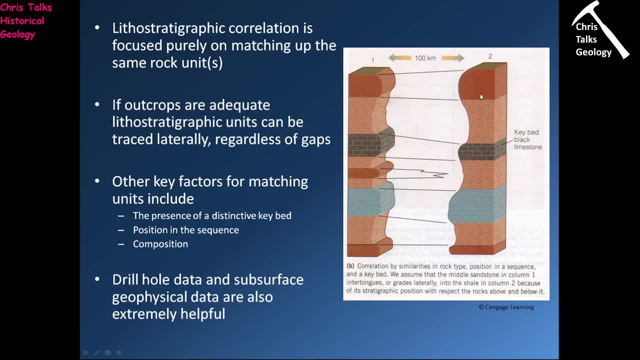 So the composition may change laterally. But if you really need to try and link the rocks together based on the composition, it's a dangerous thing to do but you can do it. So if you say right this, you know this sandstone here has a very distinct composition. 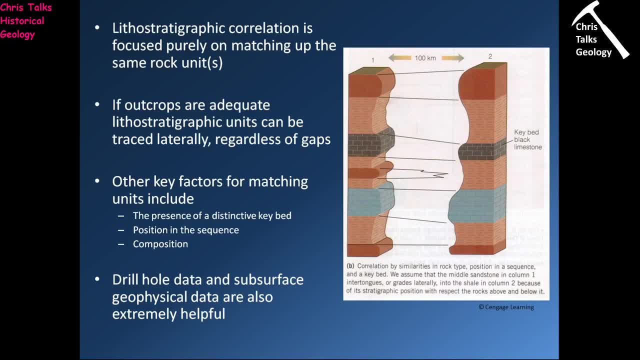 Maybe it's, you know, 95% Sand and 5% feldspar. Well then, if you come over to this location, here you find another sandstone- 95% sand, 5% feldspar. You can say, well, there's a chance that that might be the same layer, based on the composition. 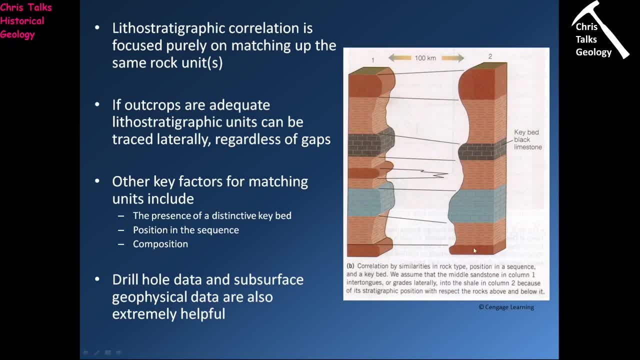 But it is a little bit dangerous because this layer down here could also be 95% quartz sand and 5% feldspar. So you know, you have to bear that in mind. So lithostratigraphic correlation. 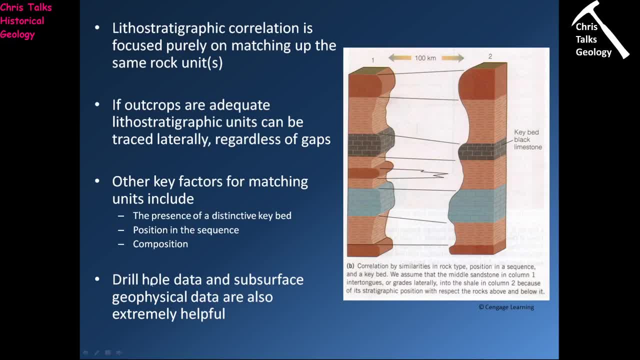 So lithostratigraphic correlations are actually also helped by the addition of drill hole data, where people take boreholes in the ground, and subsurface geophysics, So techniques like seismic surveys will allow you to track layers of rock in the subsurface. 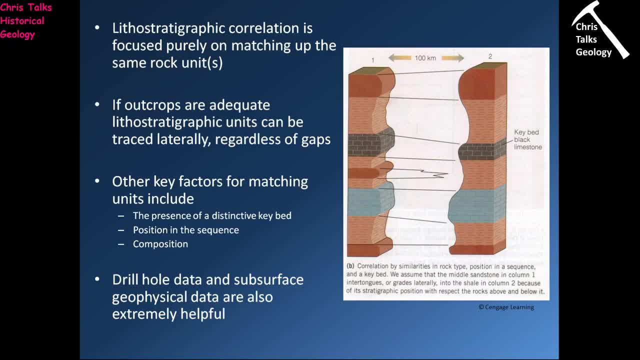 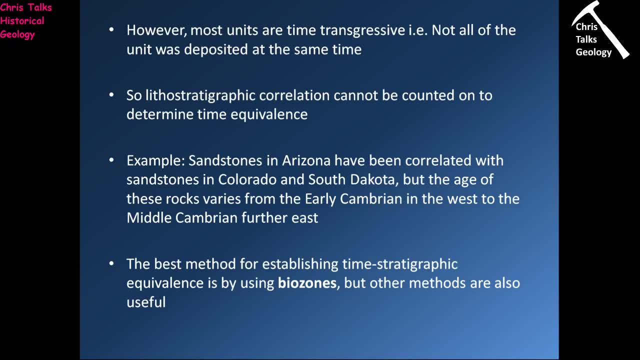 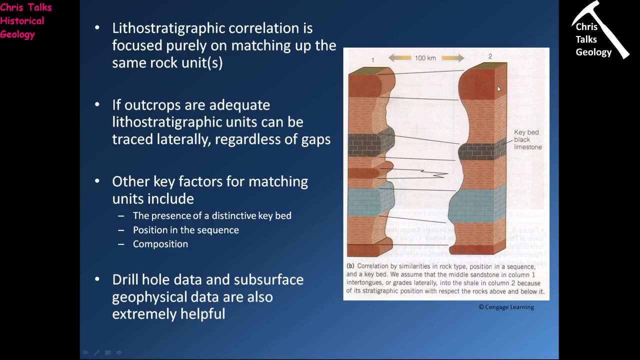 And so this allows us to do these lithostratigraphic correlations over large distances. However, we do have a problem. Most rock units are time transgressive, So, if you remember, that's a problem. So that means the age of this unit is going to change as we move laterally. 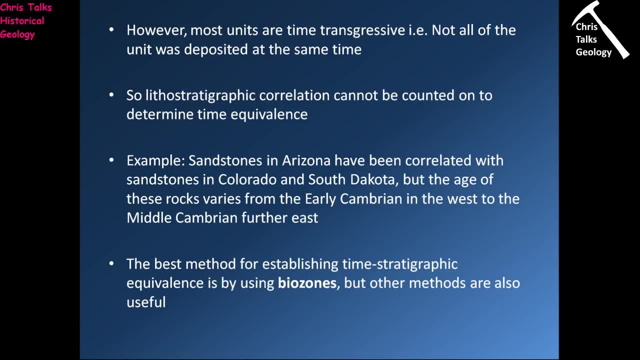 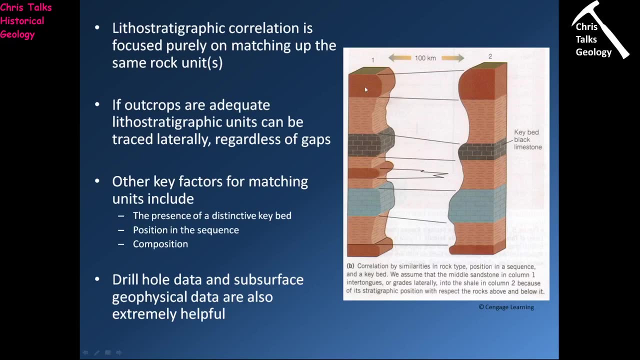 You'll get older in one direction and younger in the other direction, So lithostratigraphic correlation cannot be counted on to determine time equivalence. So if we just go back to the previous picture here, just because they're the same layer of rock doesn't mean that the sandstone at location one is the same age as the sandstone at location two. 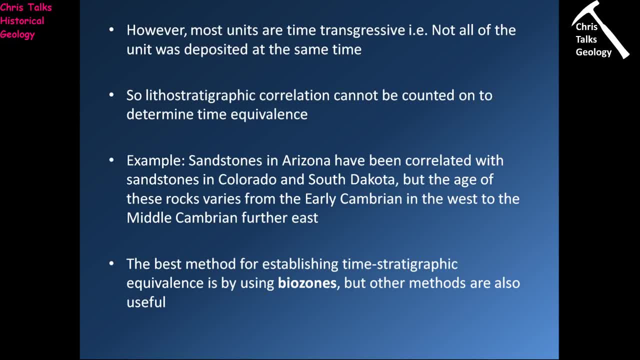 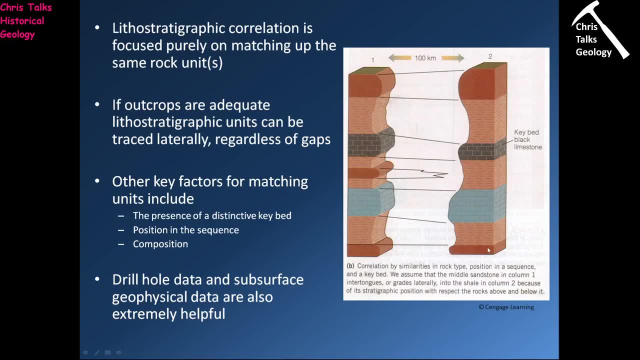 So obviously this is a bit of a problem. So lithostratigraphic correlations are absolutely great if you just want to follow a layer of rock. So if you're in the oil industry and you know this mud, So let's, let's say for argument's sake this: this mudstone here producing is very organic, rich. 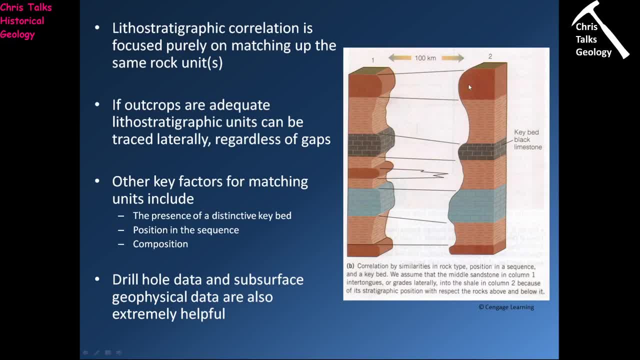 It produces oil. The oil and gas moves up into the sandstone here, which will be your reservoir rock, The rock that contains the oil and gas you want to pump out. So obviously, if you're in the oil industry, you're concerned with the lithostratigraphic correlation. 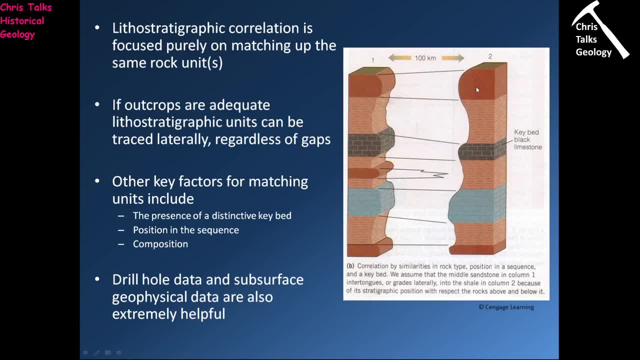 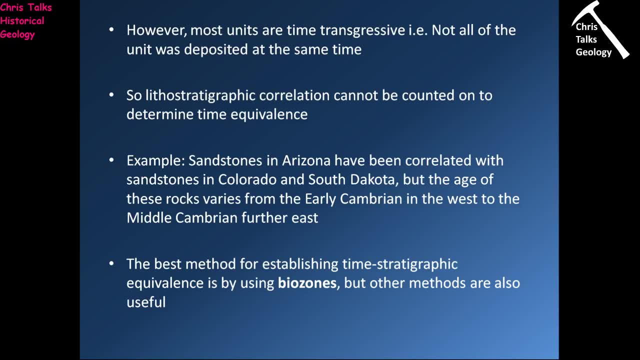 I'm just trying to follow The layer of rock. you don't really care about its age. But if you're trying to keep track of the age of your layer, if you're trying to keep the age of the rock- and you don't really care about what the what the rock is- you have to use a time stratigraphic equivalence. 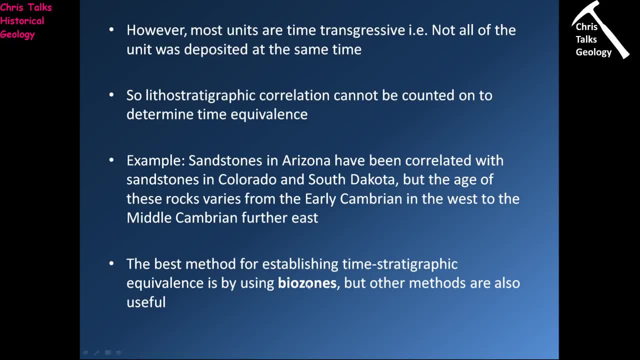 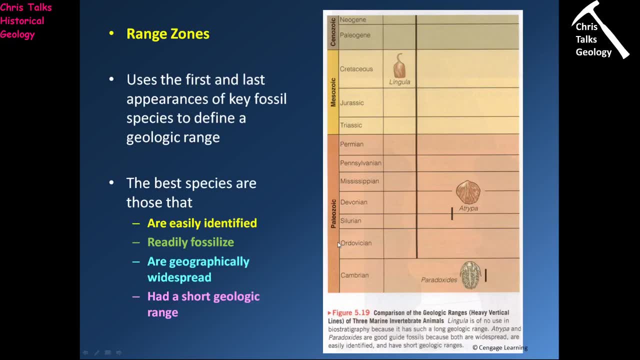 So you're going to have to use fossils and absolute age dating. So we're coming back to the bio zones now that we spoke about a few slides ago. So the first thing we can do is we can use fossils to define what are called. 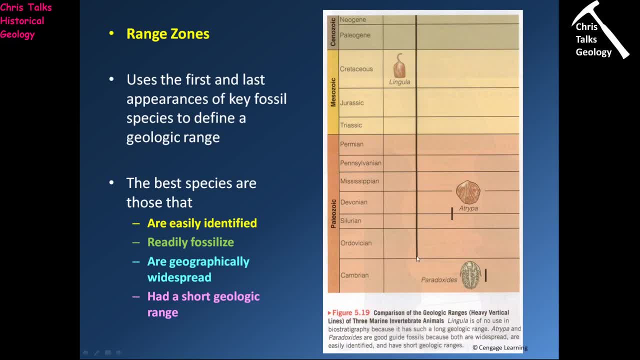 Range zones. So a range zone is the period of time between a fossil first appearing and a fossil last appearing. Now, as you can see, some organisms will have large range zones and some will have quite small range zones. So something like paradoxities down here, which is a type of trilobites you can see. it existed in the middle Cambrian. 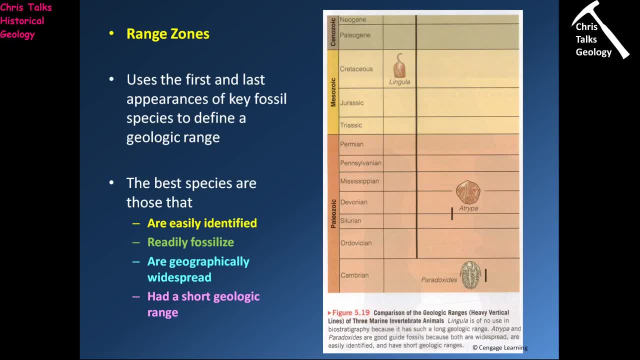 Now this is great because if I can find paradoxities in my rock, that tells me straight away that that rock Must have formed in the middle Cambrian. In contrast, lingual here is absolutely useless in terms of being arranged and because, look, it starts here in your division about 480 million years ago. 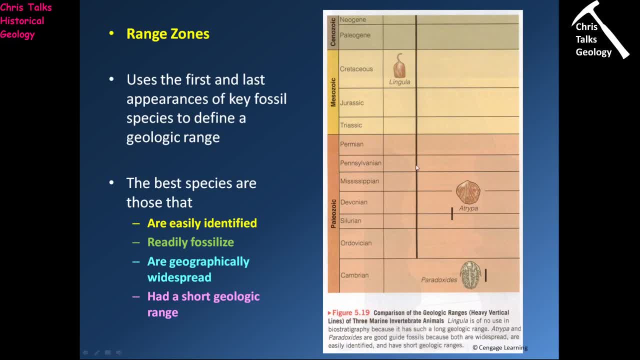 And it's still around now. So that means we can you know, if we find a rock that contains a lingual fossil, it could date anywhere between the division and the present day. So, when it comes to defining range zones, what fossils do we actually want? 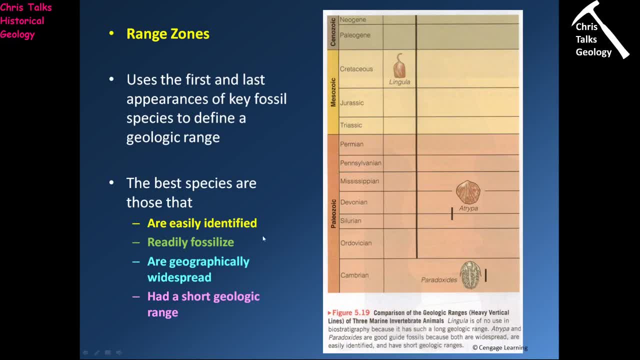 Well, the fossil. The first thing is that we want our fossil to be very easily identifiable. So, you know, when it comes to paradoxes, most even, you know, quite quite regular geologists like myself can identify it in a rock quite easily. 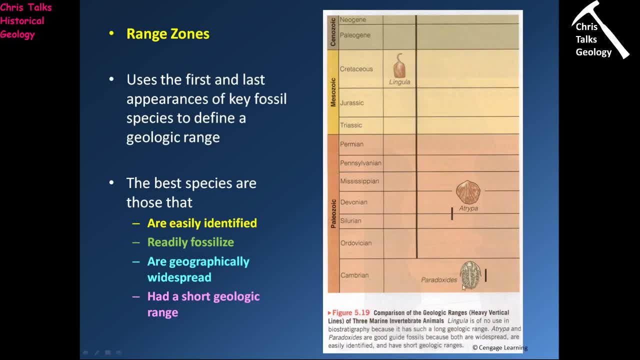 So you know, it's a nice, easy, easily identifiable fossil, So it's good for dating. We also want our organism to readily fossilize. That's also very helpful to us. The more fossil and the more examples of it we have, the easier it will be to find. 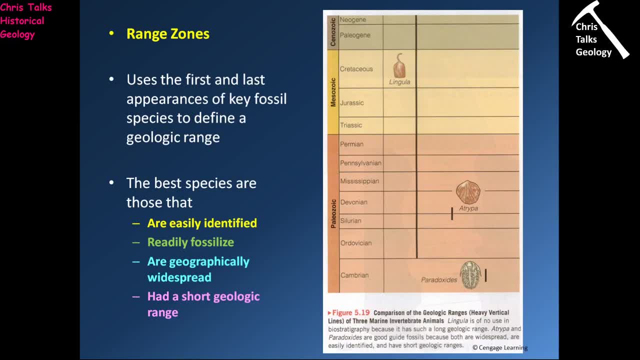 We also want our fossil to be geographically widespread. So you know, what we really want is we want a fossil that occurs in the rocks of the United Kingdom but also occurs in the rocks of Western Russia, for instance. You know, if I have a fossil that occurs in, you know, Houston and we see it in Dallas, but it doesn't occur anywhere else. 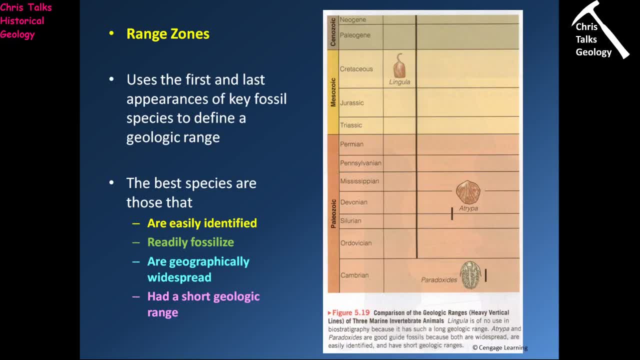 Well, that's OK if you're trying to link the rocks together between Houston and Dallas, But as soon as you go anywhere else, it's completely useless, isn't it? So what we really want is we want a fossil that was everywhere. 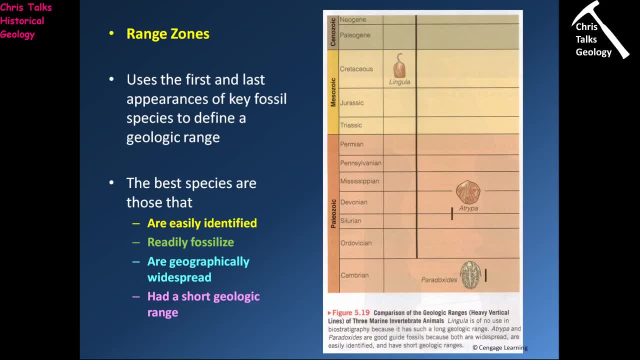 The more widespread the better. And the final thing we want is we want our fossil, our organism, to have had a short geologic range. We want it to have appeared and then disappeared from the geologic record quite quickly, Because the smaller the range, the more accurate the dating can be. 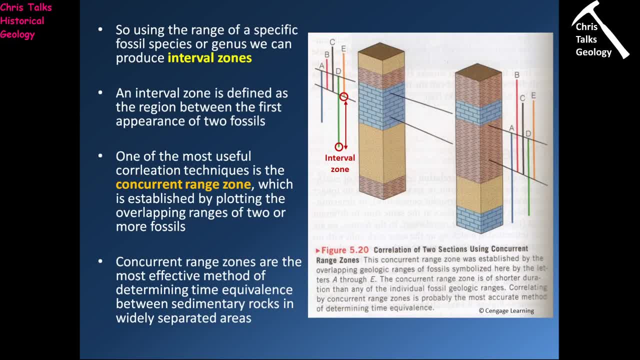 So what we can do is we can use these range zones to define. So we can use these range zones to define a couple of different units, or should I say zones. The first type of zone we can define is an interval zone. So an interval zone is defined as the region in the rock record between the first appearance of two fossils. 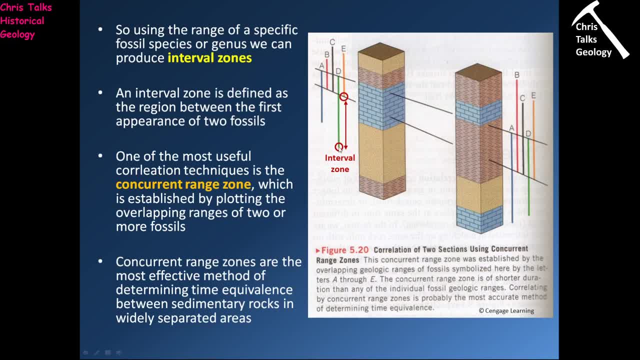 So on this diagram here I've defined an interval zone So we can see: fossil D makes its first appearance here, Fossil E makes its first appearance there, So we can use the package of rocks from here to here And we can use that. 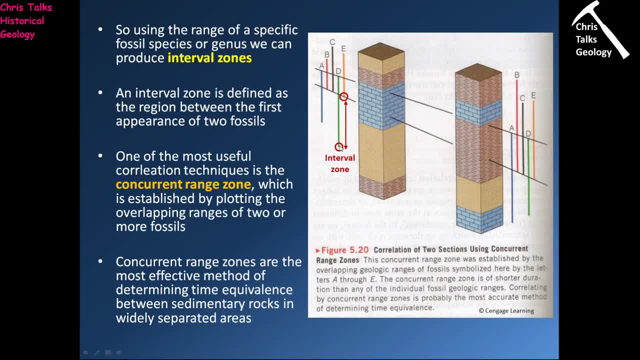 And we can use that to define an interval zone, Because fossil D appears, fossil E appears. That's going to be our interval zone, So the interval zone is just selected pretty much randomly. Now that's helpful to some degree, So we can use interval zones to correlate rocks over large distances. 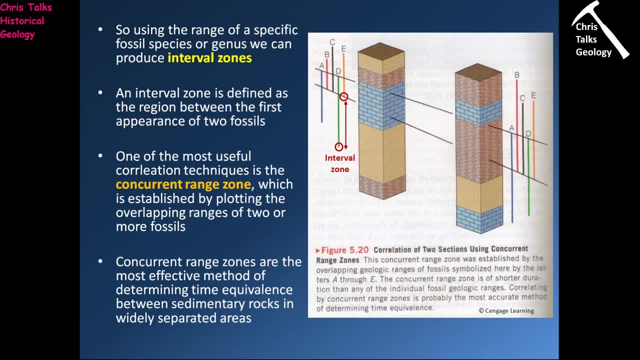 But the accuracy is somewhat lacking. What we really want is: we want a technique that allows us to correlate rocks over large distances, But it also has to be a technique that allows us to correlate rocks over large distances, But it also has to be a technique that allows us to correlate rocks over large distances. 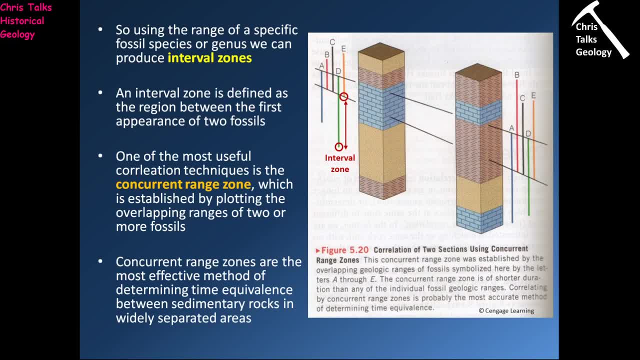 And that really gives us an added degree of accuracy. That's what we're really after, And so, in order to do that, we use what's called a concurrent range zone. So in a concurrent range zone, we take several different fossil species. 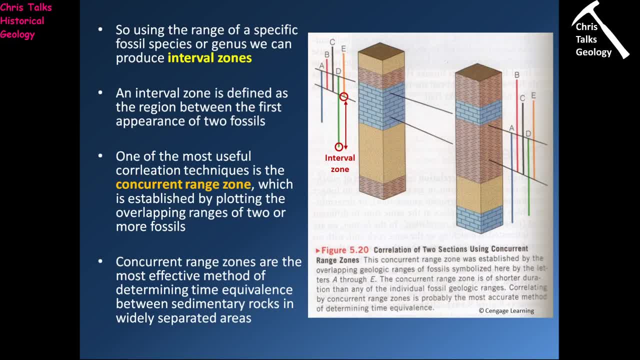 And we look for the point where the ranges for each of those species overlaps. So if we look on the diagram here, we can see we have fossils A, B, C, D and E And we can see that between these two lines that's the period of the geologic history. 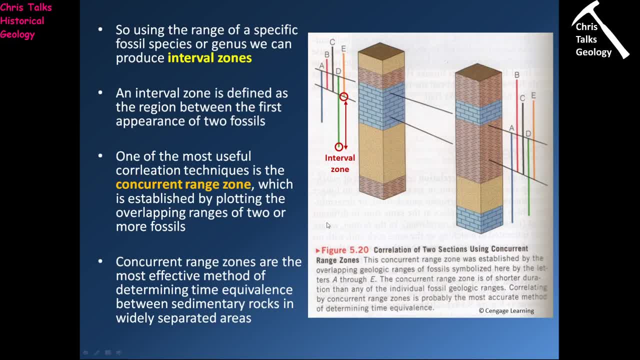 where these five fossils overlap would have all been able to live together simultaneously, and so this means if we go to another location, be it 10 kilometers away, 100 kilometers away or you know, 500 kilometers away, and we see the same group of fossils. there's a, b, c, d and e in this layer of rock here, even though 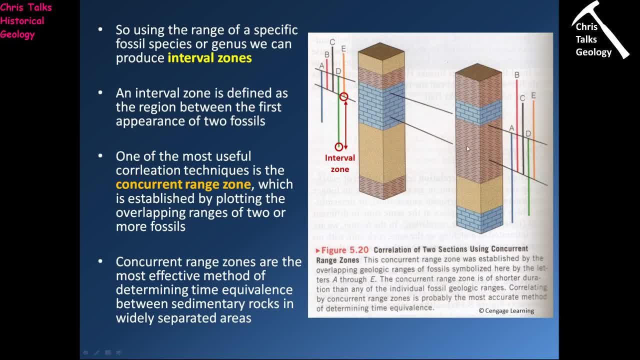 the layer of rock is different. it's a limestone over here and a mudstone over here, because it contains the same five fossils. we know this mudstone must have been forming at the same time as this limestone here. and concurrent range zones are great because you are using, you know, in some. 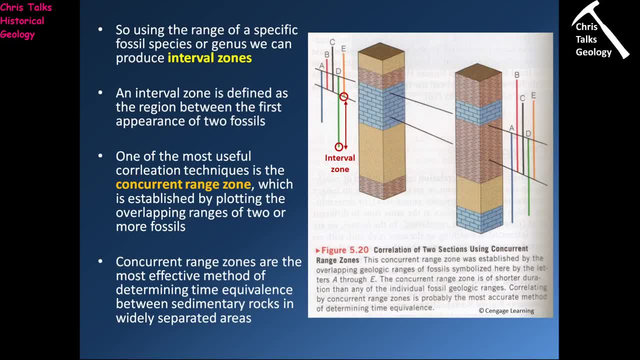 cases, you'll use maybe even dozens of fossils to to define your concurrent range zone. so it's super accurate because there will only be a very limited period of time during which these fossils will have all been able to coexist together, and so it helps to take fossils that in some cases have. 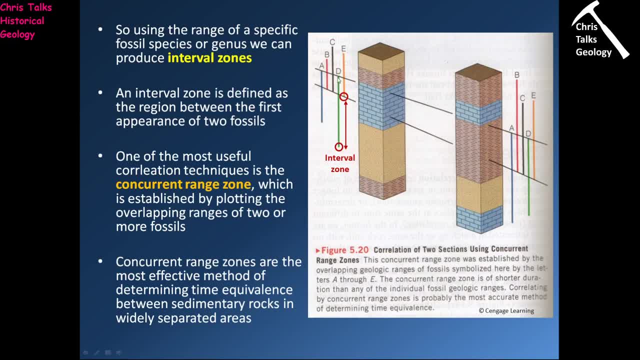 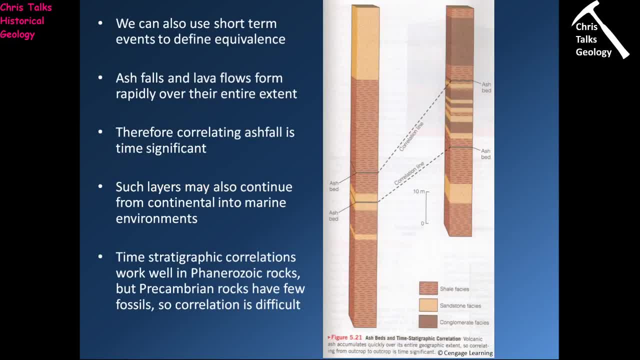 so the final technique is obviously going to be using absolute ages to produce a, a time-based correlation between layers of rock. so we can use short-term events to define the time period during which it will have coexisted with other species. so we can use absolute ages to define equivalents, so we can look for things that happened on a very 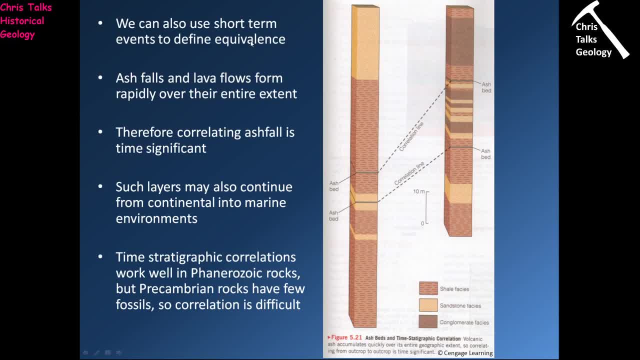 short time scale. volcanic eruptions are a prime example of that. so if you have an explosive volcanic eruption, it throws a whole lot of ash and dust into the atmosphere. wind obviously blows that ash and dust over the surrounding area and it will settle out and form a layer on the ground. 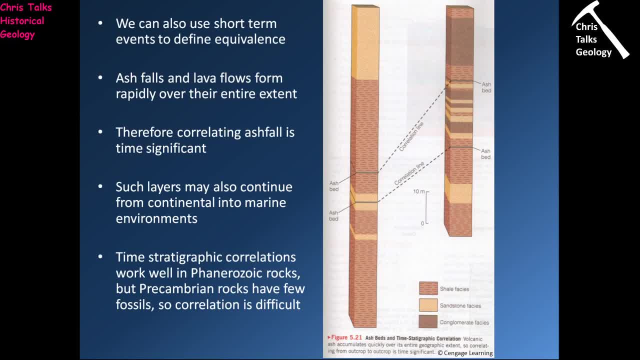 and that layer of ash can then be incorporated and turned into a layer of rock which will become part of the rock record. and so if we look at our location here, we can see that the rock record is a kind of a physical rock out here we can see we've got some mud, stone, sandstone, mud stone, sandstone, mudstone and sandstone, but within this sequence we have these two gray layers and these are ash beds. 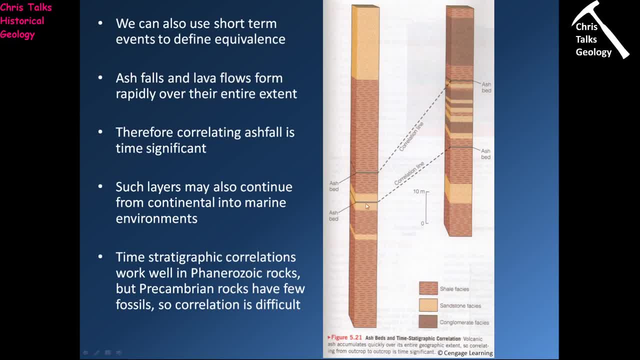 from volcanic eruptions. now, the great thing is is that these ash beds will contain minerals like zircon, which we can date, and so we can extract the zircons. we can date them through radiometric dating and we can get an absolute age. and then, at our second location, 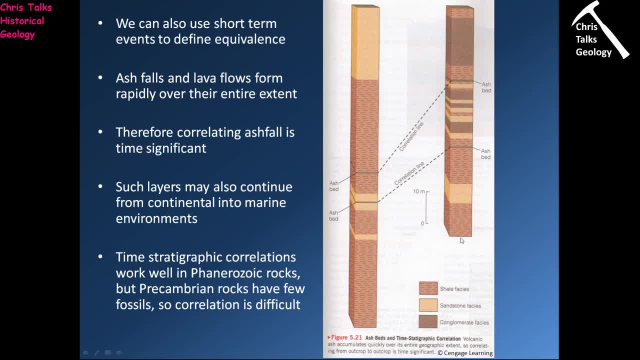 we can see, in this instance we have a completely different sequence of rocks. we have in this case mudstones, sandstones, but we also have some conglomerates as well. but once again, there are our two ash layers, and so we can use the ash layer here, if we can get a date for this ash layer. 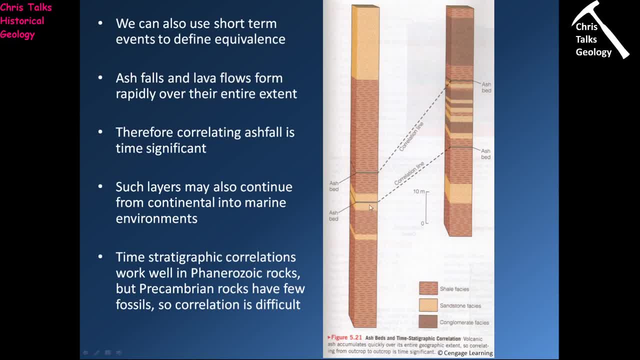 and a date for this ash layer and we saw that and we see they formed at the same time. we can correlate between them. we can say: right, this layer and this layer were produced by the same volcanic eruption, then the same goes for this layer and this layer. so, as long as we can, 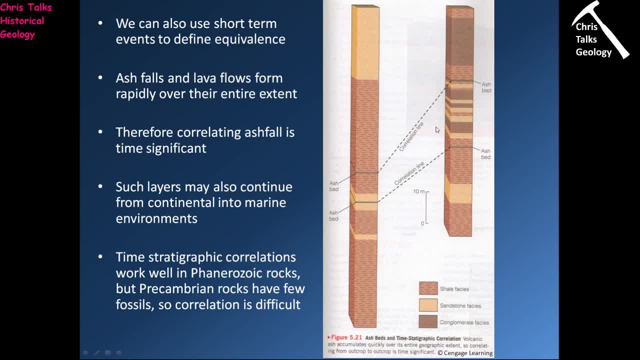 date the layer to get a numerical value. we can use that to correlate between them. now, in terms of things like ash layers, they are only effective in a local area. most volcanic eruptions do not produce a layer of ash which covers a large area. okay, the only example of 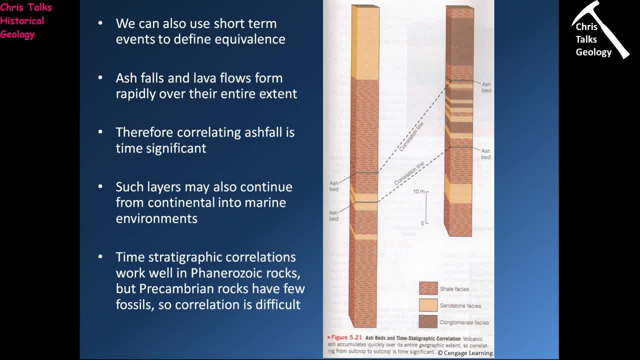 an event that's produced a layer of ash which is extremely laterally extensive. was the kt impact at the end of the cretaceous. that produces a, that produces a layer of um, of what's now clay, but was ash which covered the entire earth. so if you go pretty much 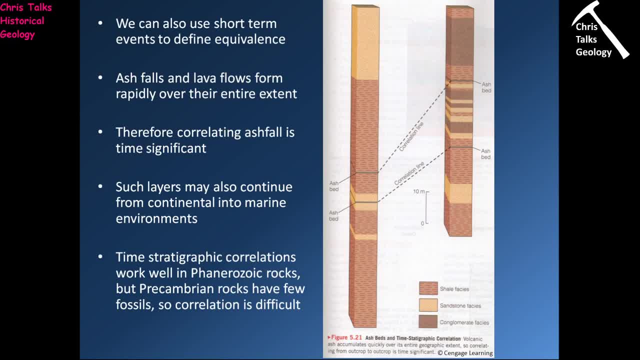 anywhere on the surface of the earth and you find the cretaceous cenozoic boundary, you will see there is a very thin layer of kind of white gray clay there and that represents the ejector from the impact 66 million years ago. so that's, that's the one time when you can actually use a layer. 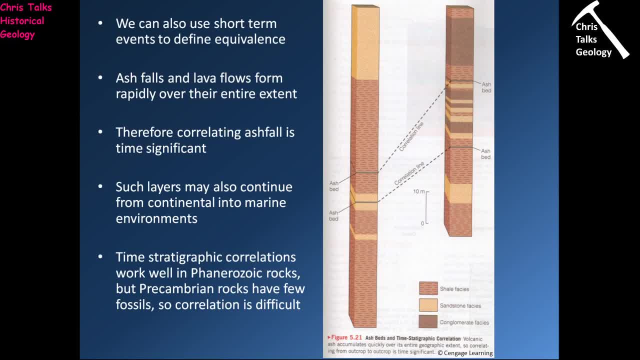 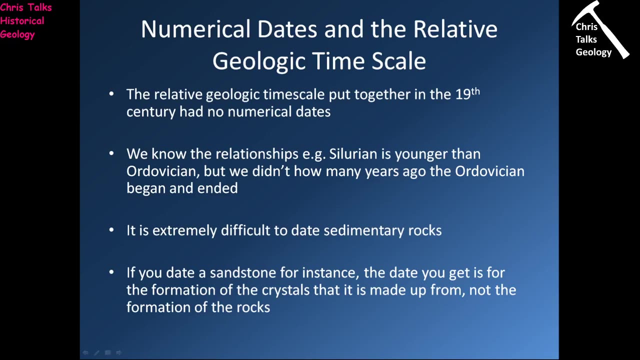 of ash to date over very, very large distances, but that is a very, very rare um thing. most volcanic eruptions will only produce a layer of ash which will cover a relatively limited area. so the final thing we need to think about now is, excuse me- is the application of numerical dates. 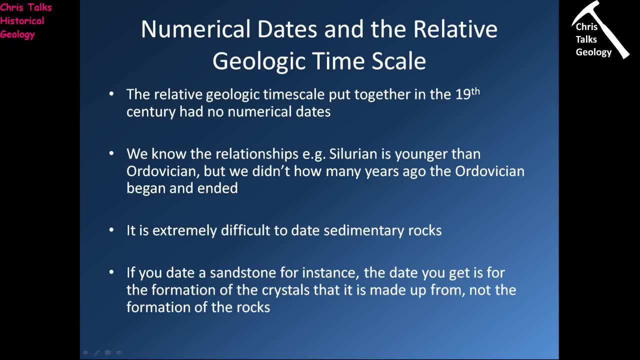 to the relative geologic timescale because, remember, the geologic timescale is essentially a relative timescale. what you're looking at is a, a sequence of systems that were stacked one on top of another based on their relative ages, and then some of the boundaries, some of the smaller. 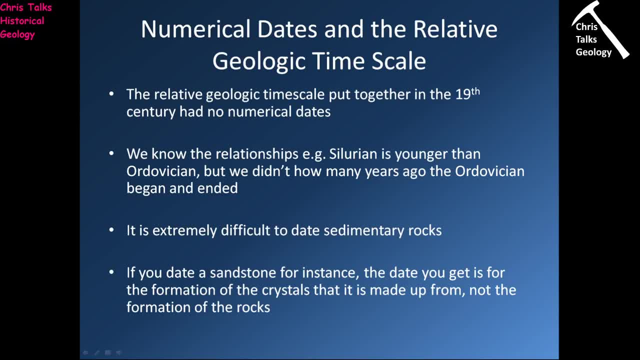 boundaries and larger boundaries we see on the geologic time scale, were defined by using fossils. so that's relative dating using fossils and relative dating using rock units. Now, as we've also discussed, since the 1940s we've had the capacity to date rocks radiometrically, so that 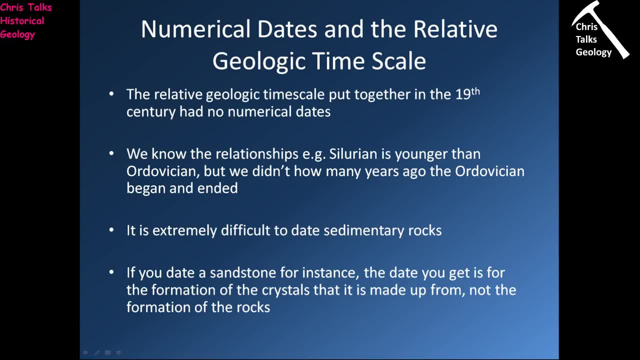 has meant. over time we've been able to add numerical ages to most of these boundaries, so you know how are we going to do that. So it's extremely difficult to date sedimentary rocks. that's a problem that we have. so, sedimentary rocks, when you date them, especially if they're 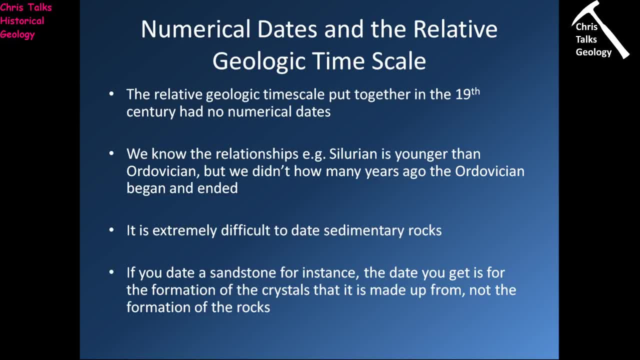 clastic. the date you're getting is not the date for when the rock formed. what you're getting is the date for when the clasts that were formed were formed. So that's a problem that we have So sedimentary rocks when you date them. 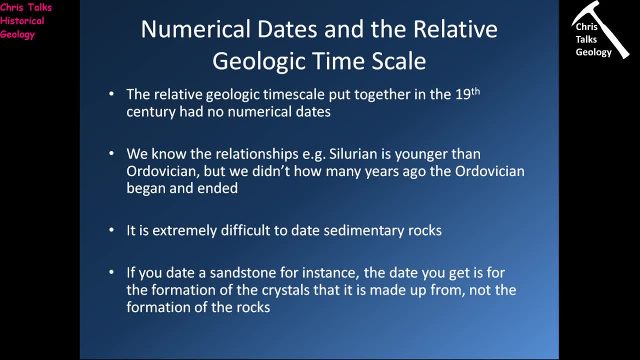 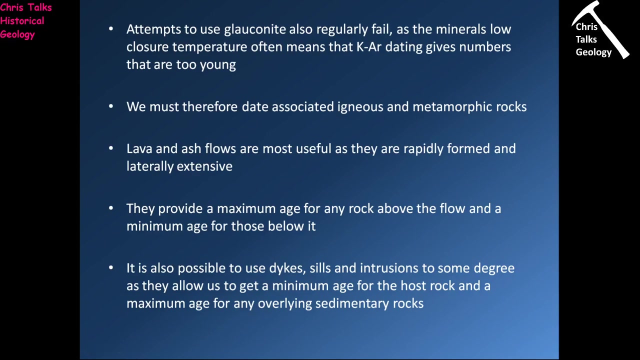 make up the rock formed. So if you have a sandstone and that sandstone was produced from a weathered granite, when you date that sandstone you don't get a date for when the sandstone formed. you'll get a date for when the granite formed. So there are some instances when you can do. 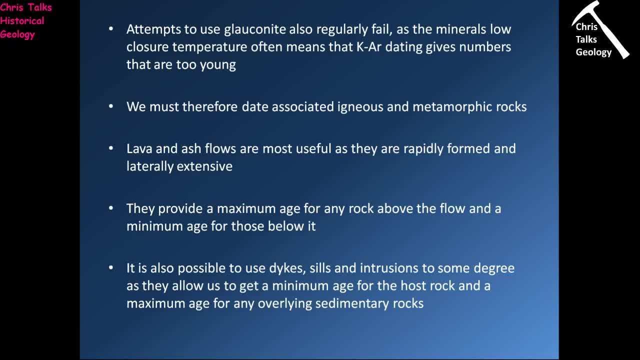 radiometric dating of sedimentary rocks. so you can use a mineral called glauconite in some instances to date sedimentary rocks. however, it is a very inaccurate dating method because the mineral itself has a very low closure temperature. so, if you remember, the closure temperature is the temperature at which if we bring our mineral above the closure temperature. 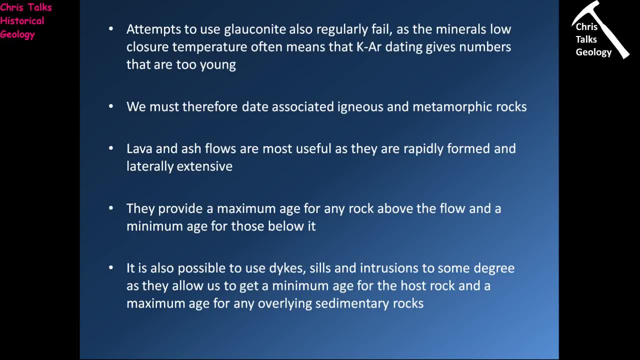 it can lose parent or daughter isotopes and thereby change the age that we get when we analyze the crystal. So glauconite can be used to date sedimentary rocks, but those rocks typically have to be quite young and they have to be in pristine condition. 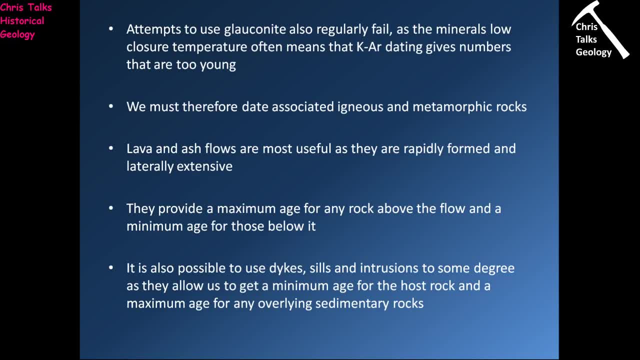 If they've been mucked about with in any way, chances are the age you're going to get will not be correct. So, when it really comes down to it, dating rocks, in order to get numerical values for the geologic time scale, has to rely pretty much on igneous and metamorphic rocks and to 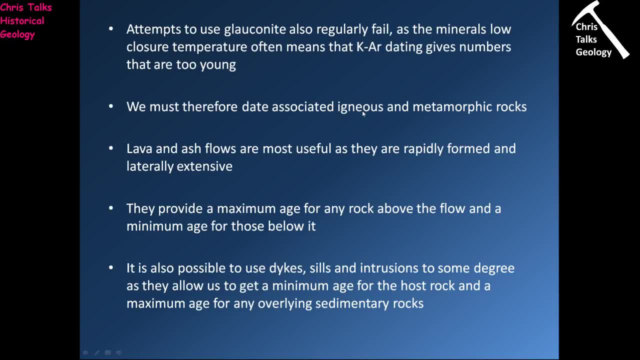 be brutally honest, igneous rocks are the ones we really want. So what we, what we're looking for in particular, are lava flows and ash flows, because they are rapidly formed and in some cases, they can be laterally extensive. they can cover large areas. So what they'll do is they'll provide a 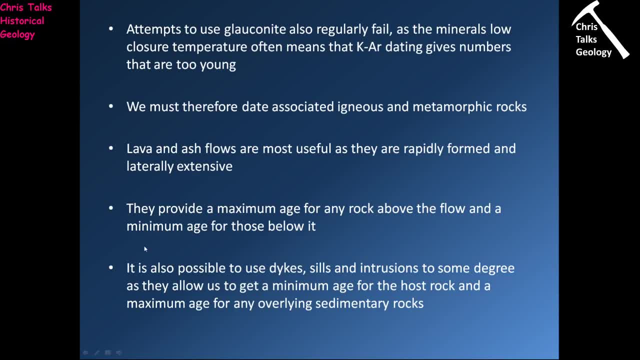 maximum age for any rock above the flow and a minimum age for any rock below the flow. So as long as we can date the lava flow, we know, while the rocks beneath the lava flow must be older and the rocks above the lava flow must be younger and we have a numerical value which we can apply to that. 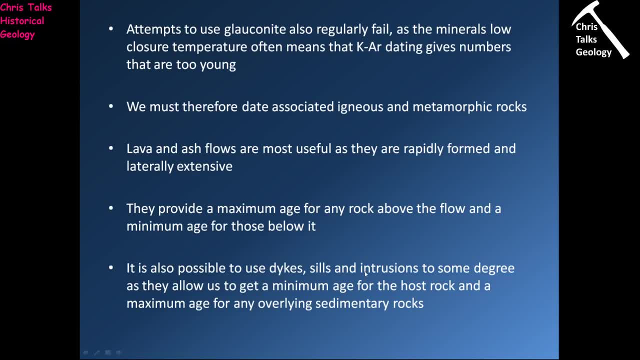 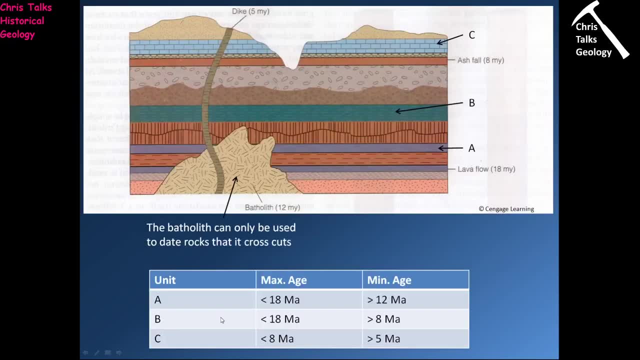 It's also possible to use dikes, sills and intrusions to also help us get an age range for layers of rock. So this diagram here is taken from the textbook, and now I would ask you to please take a minute and really concentrate on this point, because there's a good chance. a diagram like 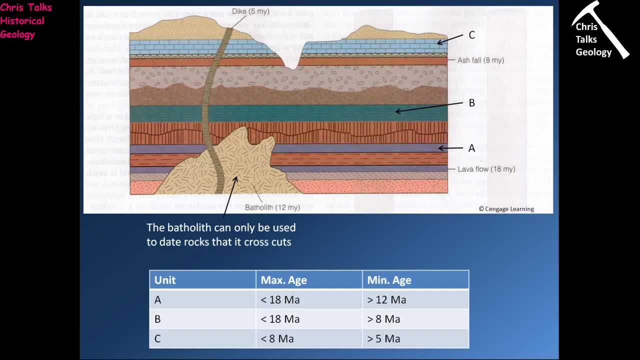 this may well turn up in the test at some point. you have been warned. So what you can see is we have ourselves a sequence of rocks here, and we can see we have a lava flow, which is this purple layer, which dates to 18 million years. we have an ash, an ash fall layer, which is this kind. 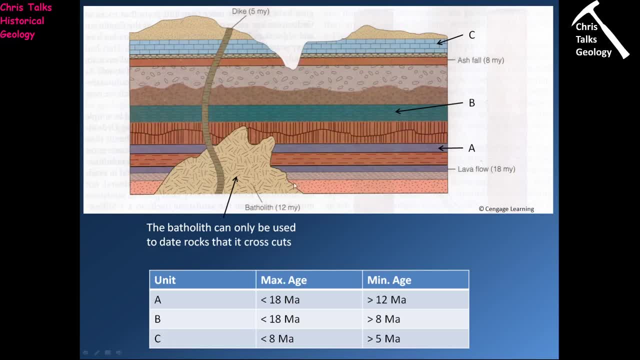 of brownish layer that dates to eight million years. we have an intrusion, a baffle lift, that dates to 12 million years and we have a dike here that dates to five million years Now, because those four layers, the ash, the lava flow, the intrusion, the dike- are all igneous, we can date them. 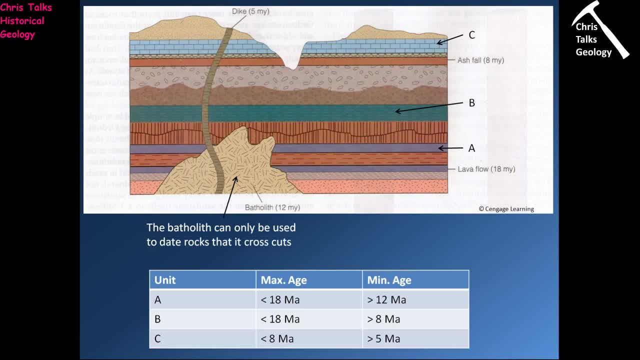 radiometrically, and we can get absolute ages, and so what we can do, then, is we can use these absolute ages to help constrain the age ranges for our layers of rock. so let's think of layer A here. well, we know that layer A sits above the lava flow, which is 18 million years old, so we know, therefore, that layer 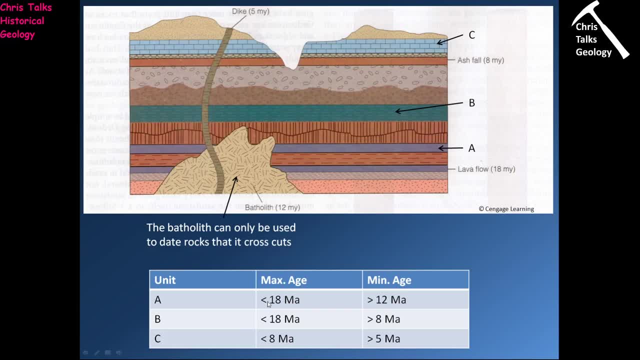 A must be younger than 18 million years. we can see, though, that layer A has been cut by the baffle lift, which is 12 million years old. so we know, therefore, layer A must have been present before the baffle lift intruded. The baffle lift must have formed after layer A, so we know that layer A must therefore be younger than 18 million years old, but older than 12 million years old, so that's still a six million year range. so you know, it's not exactly a tight time range, but nevertheless, it has helped us to produce a age range for our layer of rock. 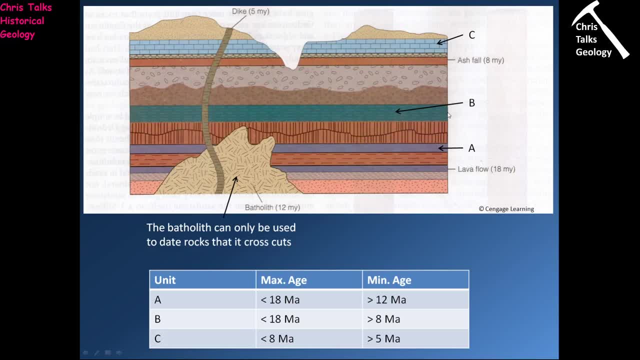 So let's think about B. so, in terms of layer B, what do we have? well, we know layer B sits above our lava flow here, so we know it's got to be younger than 18 million years. Now, the thing about layer b is it is not cross-cut by the intrusion, so we cannot use the intrusion to date. 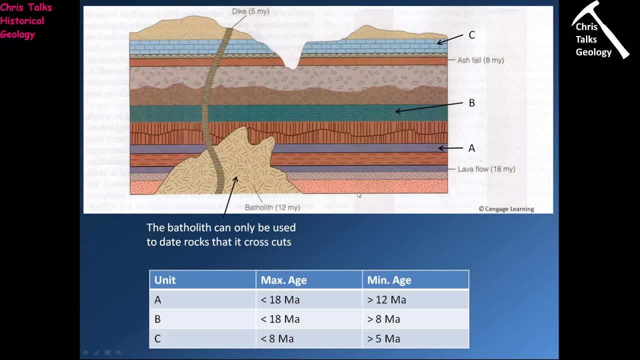 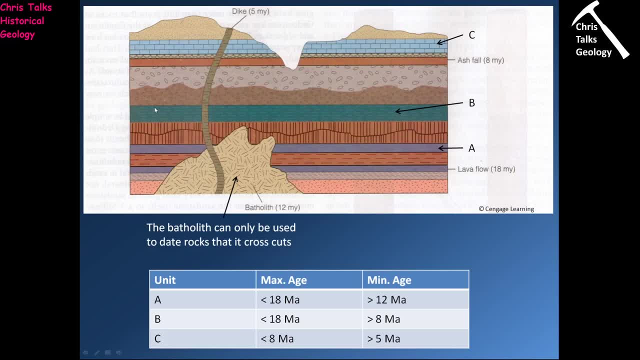 intrusion came in, then b was deposited. we just don't know the order because there's no cross-cutting relationship. So all we can do is we can say: well, b definitely formed after 18 million years, so it's younger than 18 million years, and we know well it's below the ash layer here, so we know it has. 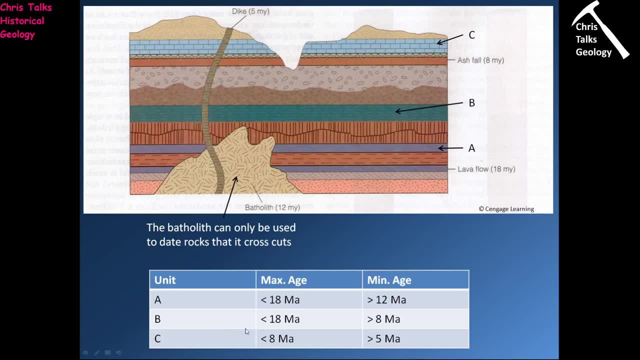 to be older than 8 million years. so we know layer b must have formed between 18 and 8 million years ago. And then, finally, we have layer c. here where we know layer c is above our ash flow, so it must be younger than our ash flow. so we know the maximum age is going. 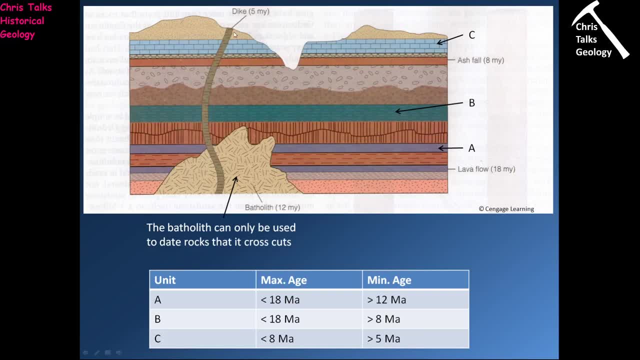 to be less than 8 million years, and we know the minimum age well. we can see here. it's cross-cut by the dike. the dike is 5 million years old. therefore, layer c must have been present before the dike was intruded, and so we know that layer c must therefore be older than 5 million years. 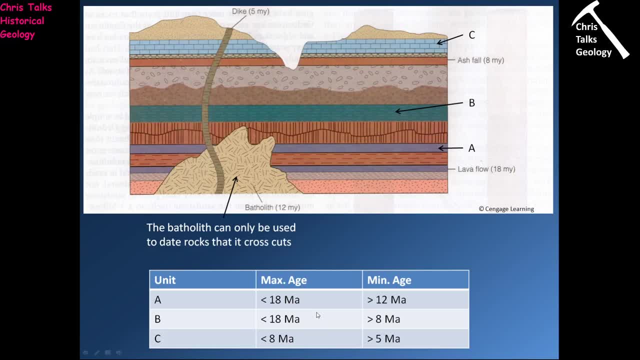 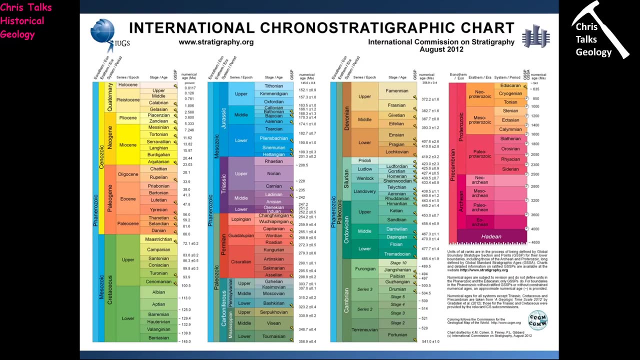 So, once again, you know these aren't super tight age ranges. I mean, you know, it's not like we're getting it down to a few thousand years- but what we are doing is we are, you know, constraining our layers and we're we're giving a time range in which they will have formed. So what we're really. 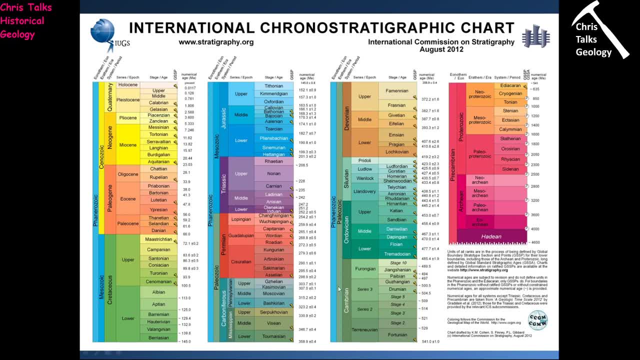 interested in, though, is the geologic time scale, so here's a picture of the geologic time scale. you've seen this before, and we know that these boundaries here are defined by the first and last and key fossils, and we also know that these dates were added later, So the question then becomes: is 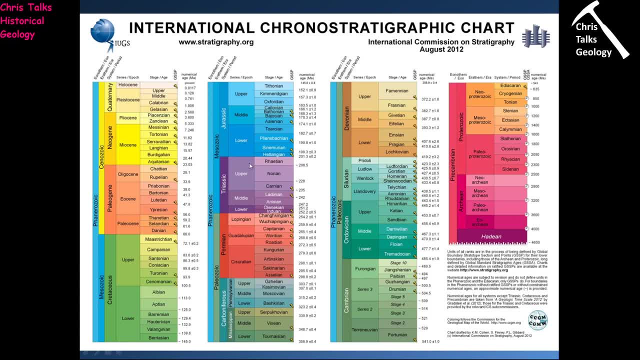 well, how do we get you know ages for these boundaries? Well, what will happen is these boundaries are based on the fossils. so what we'll do is we'll go to a location, we will look for the fossils that help us to define these boundaries and, if we are very lucky, when a fossil first or 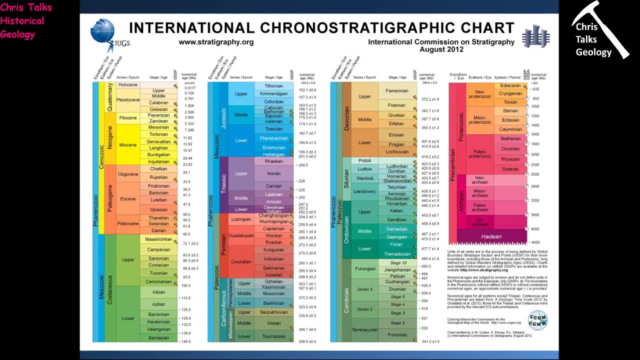 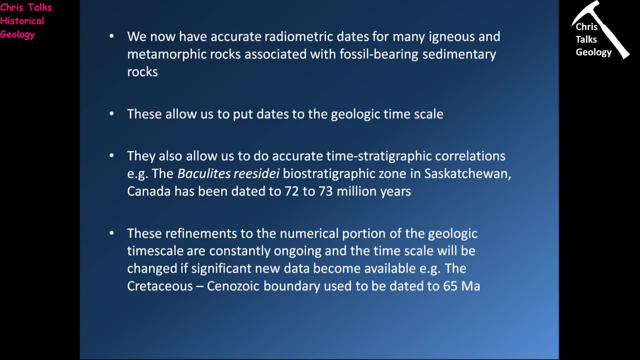 last appears one of these, you know, key fossils. if we are super lucky, then we're going to have a geologic time scale and there will be a layer of something which we can date Okay. so a good example would be what we're about to look at now. so if we have accurate radiometric dates, 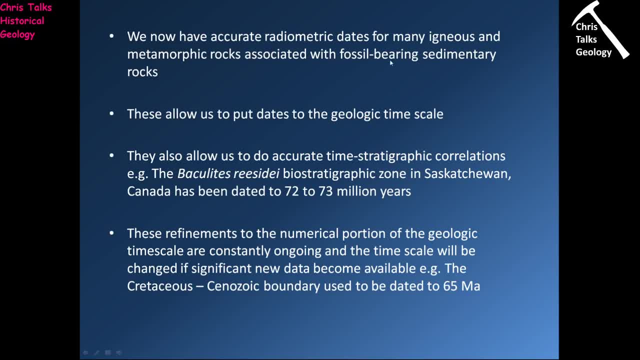 for an igneous or metamorphic rock which is associated with a fossil, we can use that to help produce an age for that fossil. So these allow us to put dates to the geologic time scale. so let's go to the next slide. so here we can see. we have a sequence of rocks, okay. 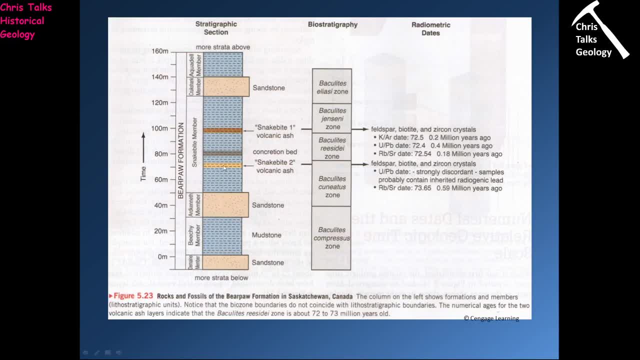 so we have sandstones, mudstones, sandstones. now the orange layer here and the brown layer here represent ash flows, so we can date these. This grey column here consists of five different species, different fossils, and you'll notice that Bacchiolites residii happens to fall almost. 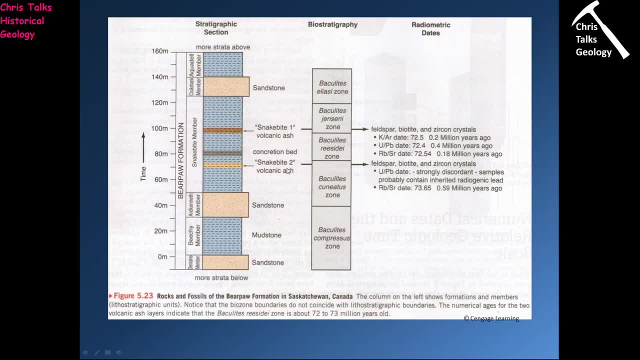 perfectly between these two ash layers, and so what we have here is we have a date that allows us to produce a maximum age and we have a date that allows us to produce a minimum age for Bacchiolites residii, So what we can see is that it existed between 73.65 million years ago. 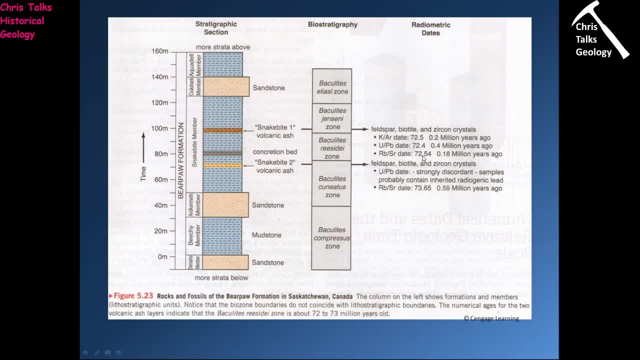 and 72.54 million years ago. give or take a little bit, and so what we have here is we have, and we have now have the ability to date this particular fossil. we know exactly when that fossil was around. we have absolute age dates to go along with it. so wherever we see Bacchiolites residii now. 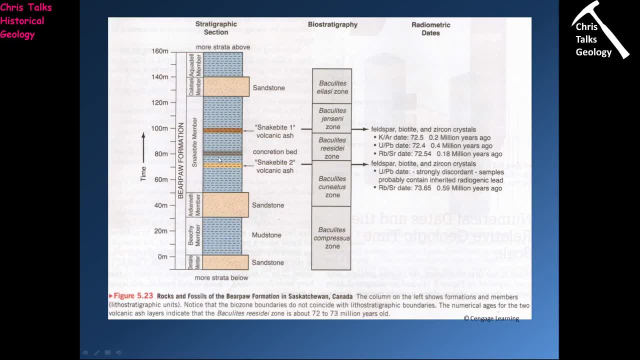 we know an exact age now, if we're super lucky, and this fossil also happens to be one of the fossils we use to define a boundary in the geologic time scale. well, once again, now we have a date for that geologic boundary, don't we? and so this is the kind of situation that we're desperately looking for, as 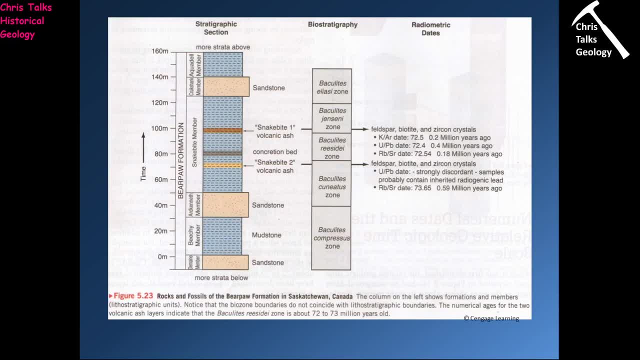 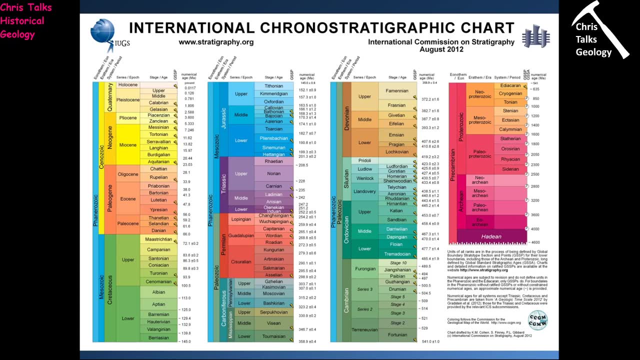 geologists to be able to actually produce an exact age for Bacchiolites residii. come up with solid numerical values for each of the geologic boundaries, and you can see that we're not doing too badly. the ones with these golden spikes here, these are the ones that we've 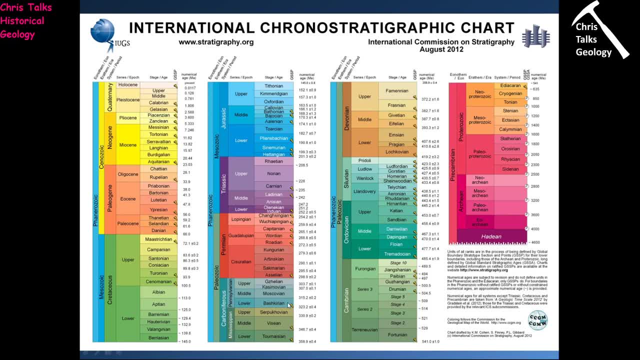 you know, really gotten you know to a high degree of accuracy, you'll notice that some of them have approximate symbols in front of them. those are the ones where we're kind of close. but you know, we haven't got it quite right. you know, maybe we have, you know the boundary and then maybe just a. 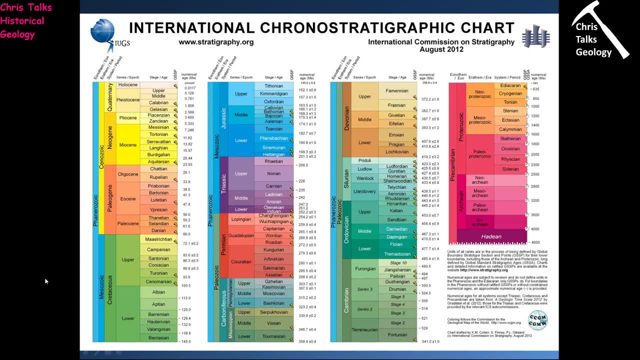 little bit above or below that. we have an ashland layer we can date. so we know, you know, the approximate age of the boundary, but we're not, you know, not- completely correct. now, if you look over here, we have the pre-cambrian rocks and 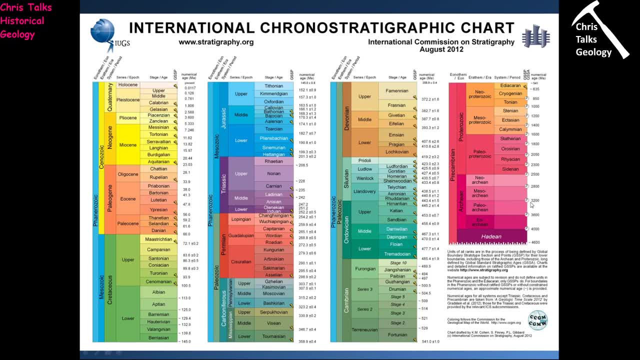 notice that they do not have essentially set dates. notice they've got these little clocks next to them. that's simply because it's very difficult to find dating evidence for these rocks, and so what's happened is geologists have just split them up into these packages. you'll notice that these 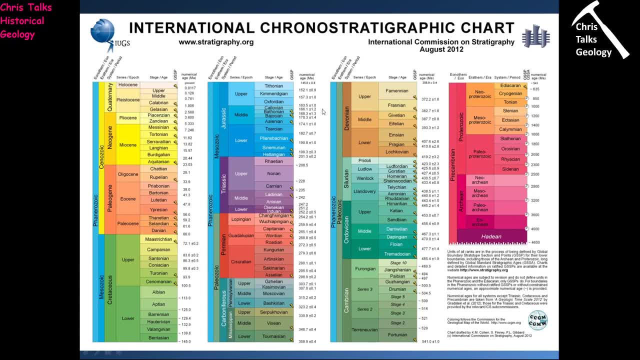 packages are all are non-existent. so you can see that these are artificial boundaries that have been inserted by geologists. so you know they're not really based on anything. attempts have been made to find dateable boundaries and we've managed to find some, but they're still not fully accepted yet. 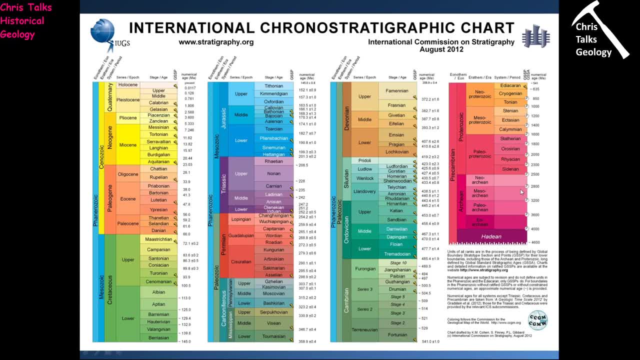 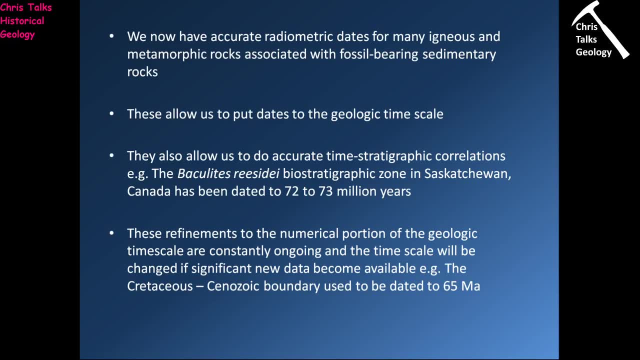 okay. so that's how we managed to use fossils and numeric dating techniques to actually produce a solid age of data. so that's how we managed to use fossils and numeric dating techniques to actually produce a solid age for different boundaries in the geologic time scale. 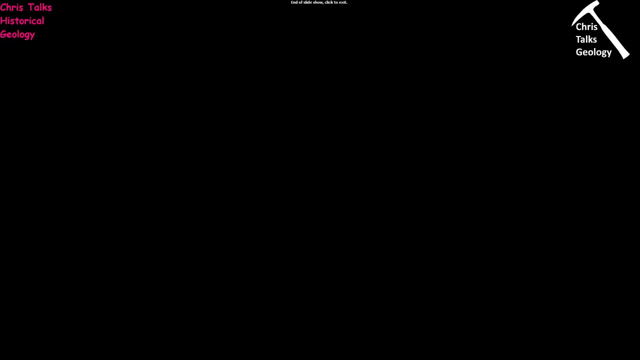 okay, everyone, so that's the end of the presentation. so thank you for listening and have a good day. 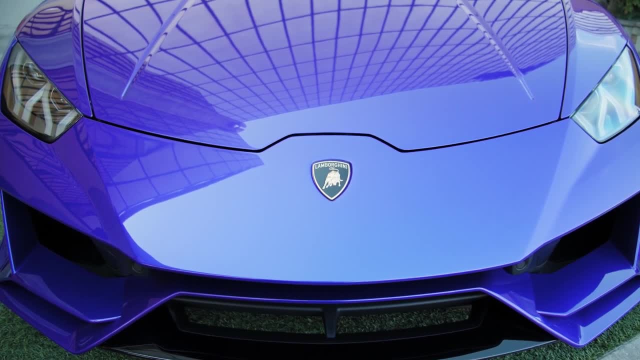 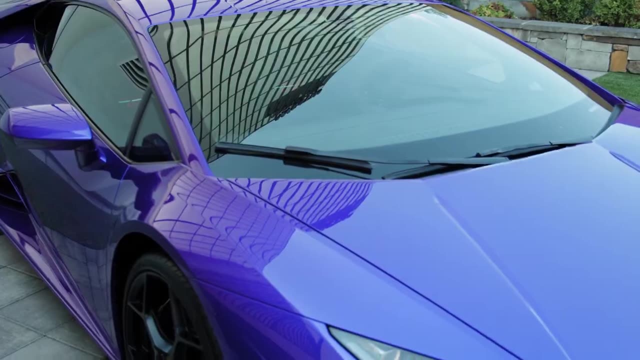 What's going on? Salutations, people. It is Lee here. What an amazing day. I have a special tour for you guys. I finally got my hands on a brand new 2021 Lamborghini Huracan. Yep, that's me. 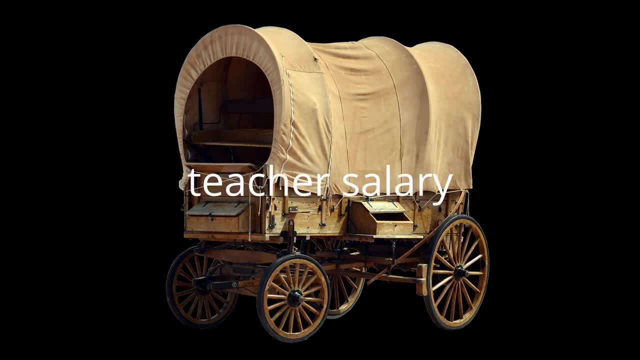 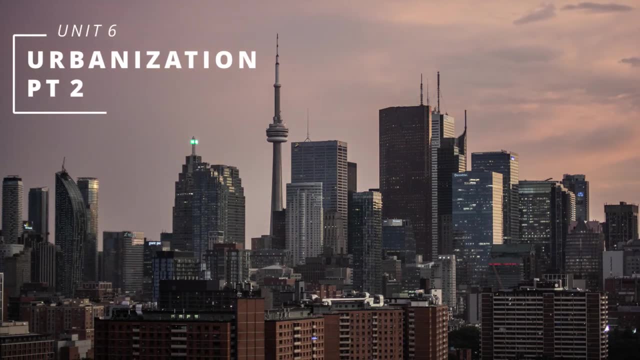 You're probably wondering how I ended up in this situation. Welcome back everyone. Mr Lee, here, And let me just clarify. my Lamborghini is actually in the shop- Standard old chain stuff. You know how it goes. So we're going to have to take a rain check. 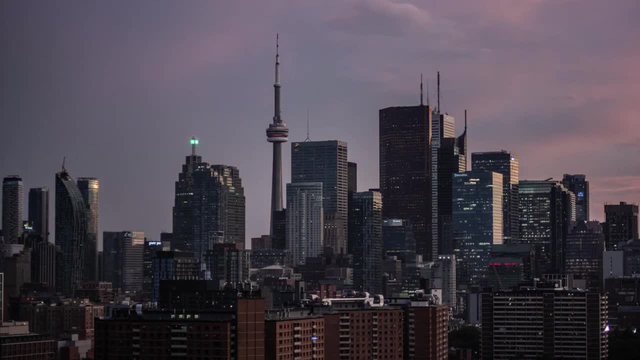 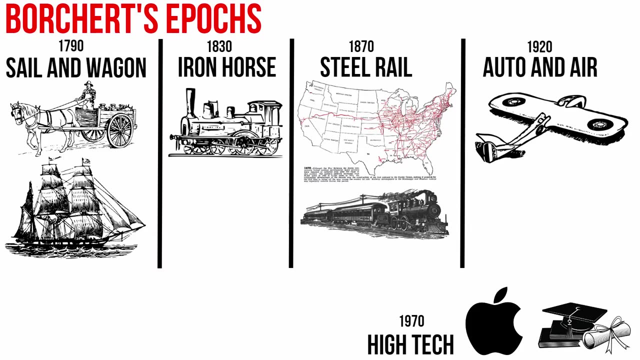 on the tour. However, if you're wondering why we're talking about Lambos and wagons, it is because we will be discussing Borchert's epics of urbanization. This model theorized that the different levels of urban development had a direct correlation with the method of 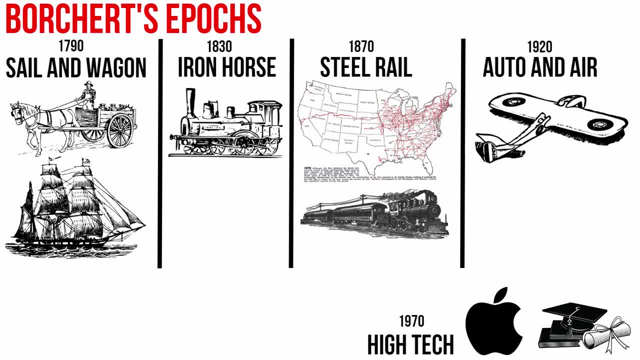 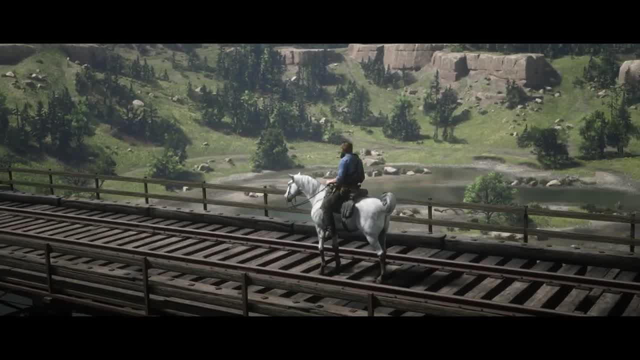 transportation that was available to the common people. And we're going to use one of my favorite games of all time- Red Dead Redemption 2, to take a deep dive into this model, as this game actually implements most of the ideas within that model. And to begin, we have the wagon and 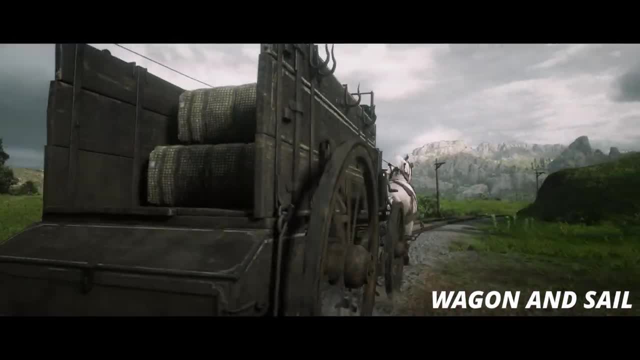 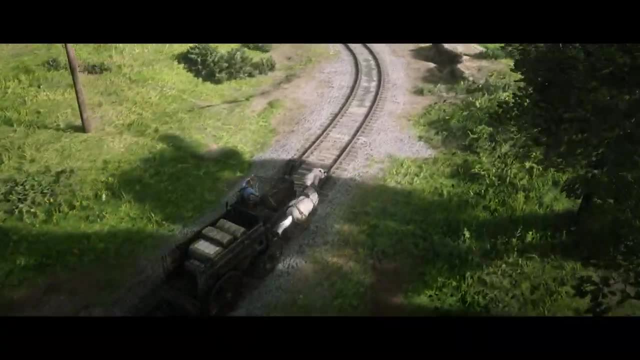 sail Epic, which said that development of cities is going to be limited within a certain radius of the CBD as methods of transportation were pre-industrial and couldn't transport people very far, And although it looks like I'm zooming over here, it was actually pretty slow Anyway.